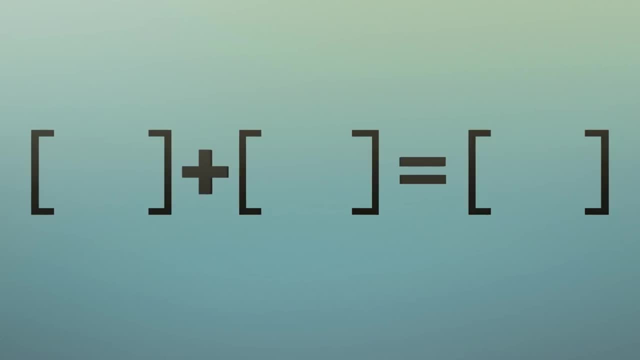 a rabbit hole of its own. Adding matrices is pretty simple. All you have to do is add the corresponding entries in the order they come, So the first entries get added together, the second entries, the third, all the way down. Of course, your matrices have to be. 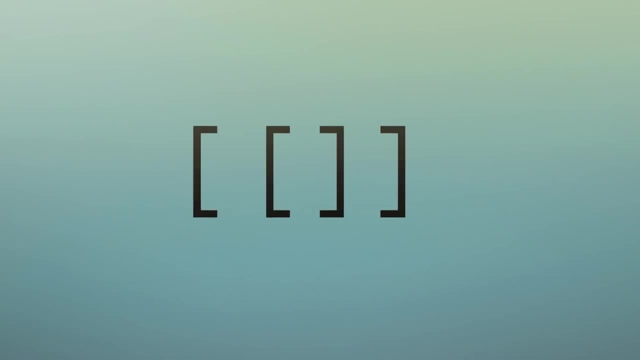 the same size. but that's pretty intuitive anyway. You can also multiply the whole matrix by a number called a scalar. Just multiply every entry by that number. But wait, there's more. You can actually multiply one matrix by another matrix. It's not like adding. 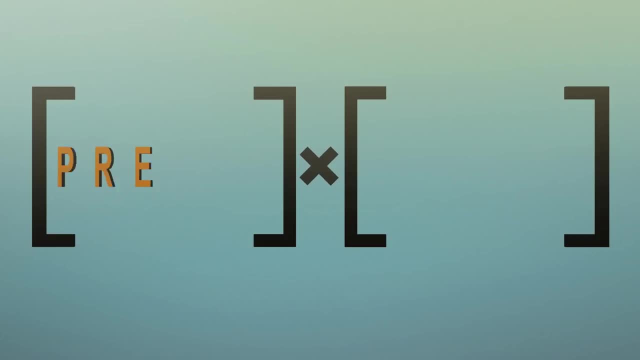 them, though, where you do it entry by entry, It's more unique And pretty cool once you've got the hang of it. Here's how it works. Let's say you have two matrices. Let's make both of them two by two, meaning two rows by two columns. Write the first matrix. 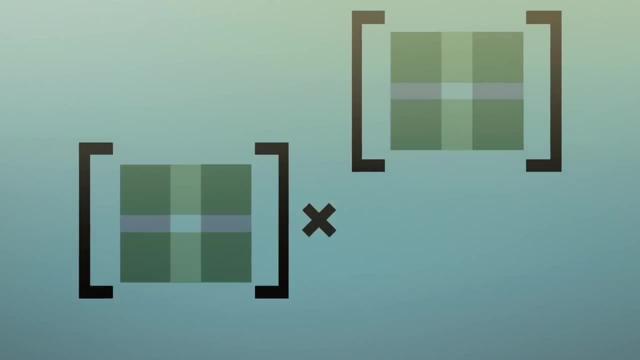 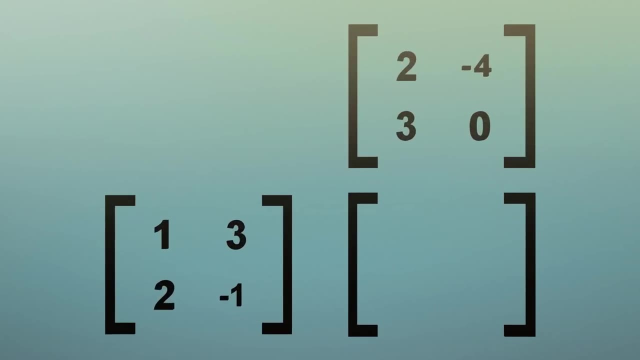 to the left and the second matrix goes next to it and translate it up a bit kind of like we're making a table. The product we get when we multiply the matrices together will go right between them. We'll also draw some grid lines to help us along. Now look, 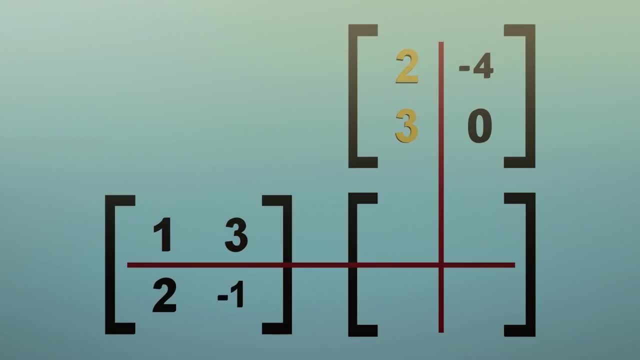 at the first row of the first matrix and the first column of the second matrix, You'll see how there's two numbers in each. Multiply the first number in the row by the first number in the column. 1 times 2 is 2.. Now do the next ones. 3 times 3 is 9.. Now add. 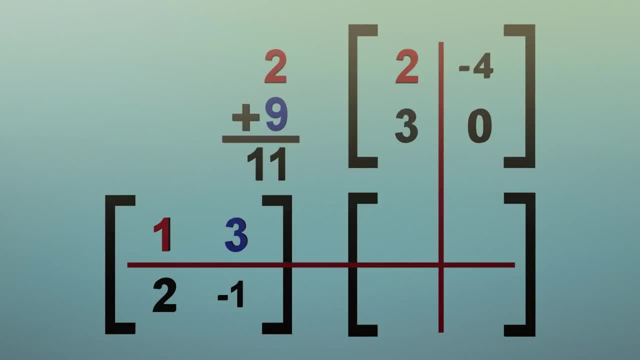 them up. 2 plus 9 is 11.. Let's put that number in the top left position so that it matches up with the rows and columns. we used to get it. See how that works. You can do the same thing to get the other entries. 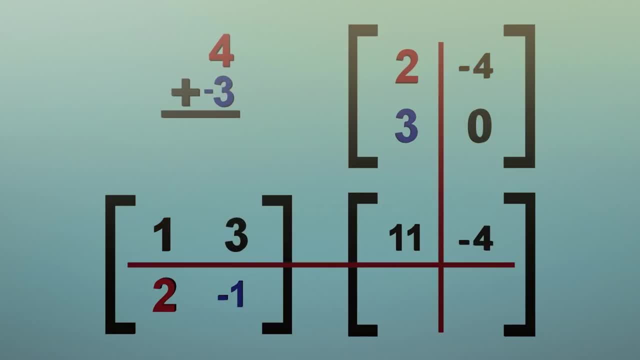 0 is negative 4.. 4 plus negative 3 is 1. Negative, 8 plus 0 is negative 8.. So here's your answer. Not all that bad, is it? There's one catch, though: Just like with addition: your matrices. 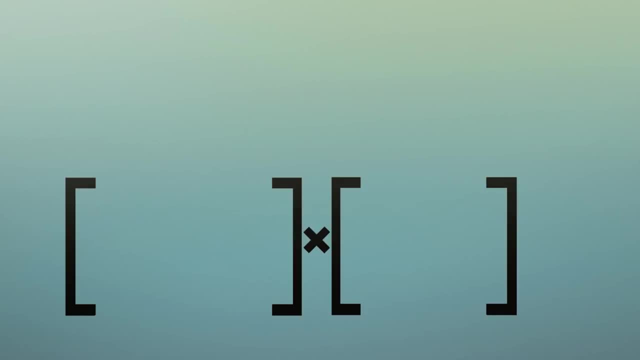 have to be the right size. Look at these two matrices: 2 times 8 is 16.. 3 times 4 is 12.. 3 times…what? Wait a minute. There are no more rows in the second matrix. We ran out of room, So.